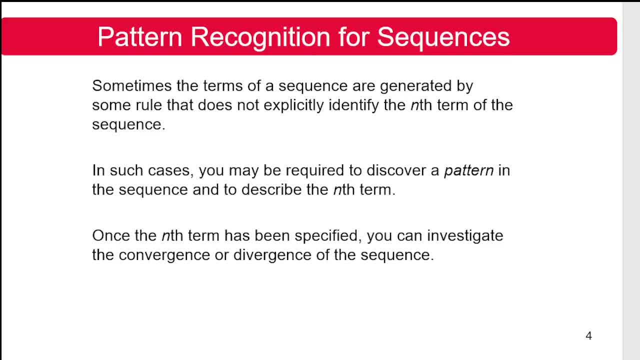 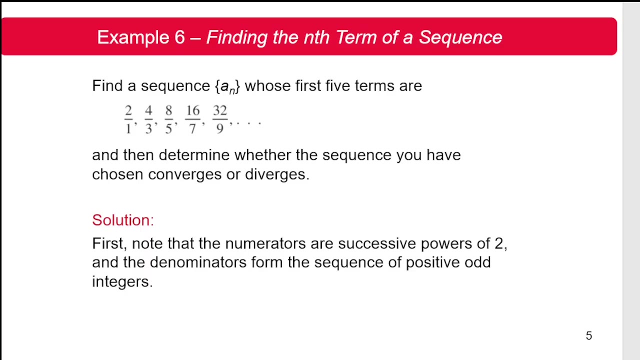 So in such cases you may be required to generate some rule or discover a pattern in the sequence and to describe the n-term. So once the n-term has been specified, you can now investigate the convergence or divergence of the sequence. Okay, like, for example: suppose we are asked to find the sequence A, sub n, whose first five 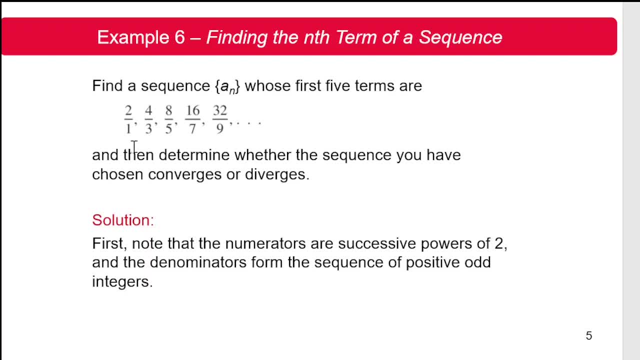 terms are given as follows: The first term is 2 over 1, the second term is 4 over 3, third term is 8 over 5, and so on and so forth. And then you are also asked to determine whether the sequence you have chosen converge or diverge. 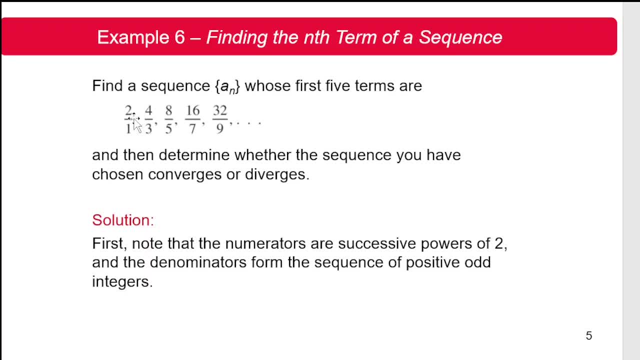 In the given sequence. as you can see, the numerators are successive powers of 2.. You have 2 to the 1, 2 squared. you have 2 cubed, 2 to the fourth and 2 to the fifth. 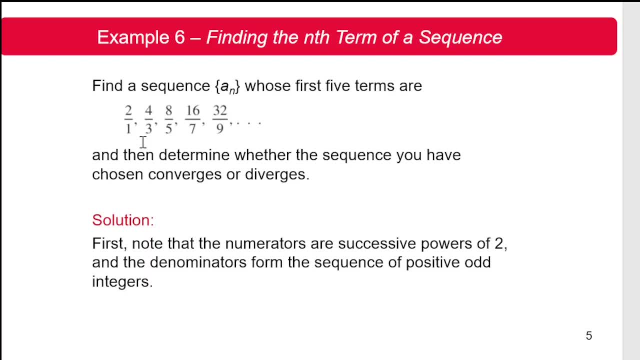 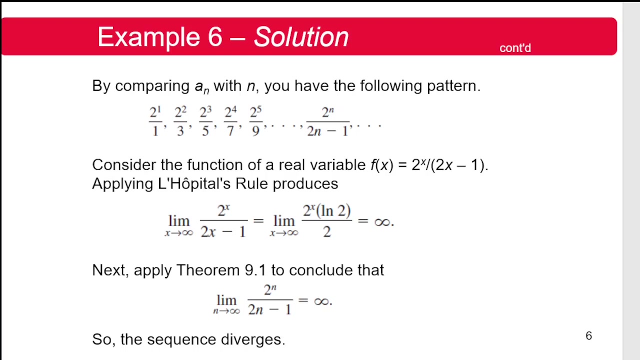 While the denominator these are positive integers starting from 1.. So from these given terms of the sequence, now we have to generate or discover some pattern or general rule. Okay, because the numerator are: add powers of 2.. So you can write this as: 2 to the 1,, 2 squared, 2 cubed, 2 to the fourth, 2 to the fifth and 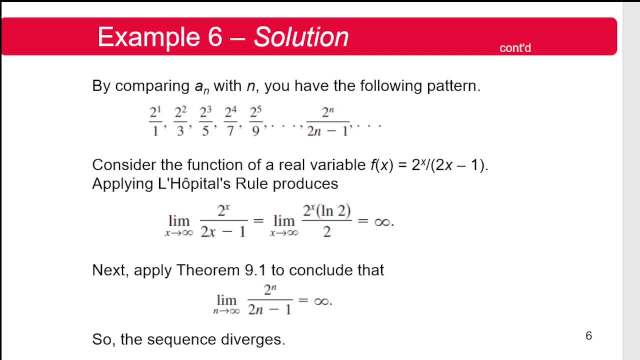 so on and so forth. So in general this is 2 to the n, While the denominator are add positive integers. So you have 1,, 3,, 5,, 7,, 9 and in general form this is 2 times n minus 1.. 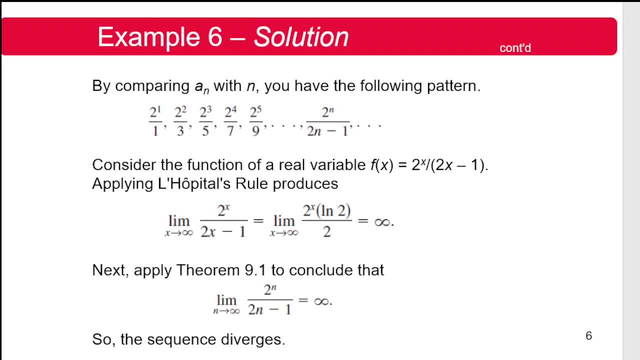 That if the value of n is 1.. So you have 2 to the 1 over 2 minus 1 or 2 over 1.. If n is 2, then you have 2 squared over 2 times 2 is 4 minus 1.. 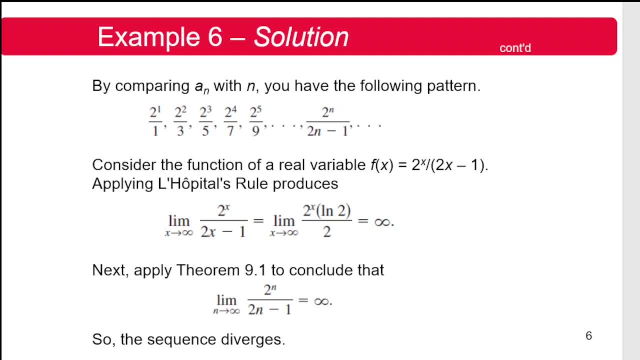 So that's 3.. So you have 2 squared over 3.. If n is 3, then you have 2 cubed over 2 times 3 is 6 minus 1.. So you have 2 cubed over 5, and so on and so forth. 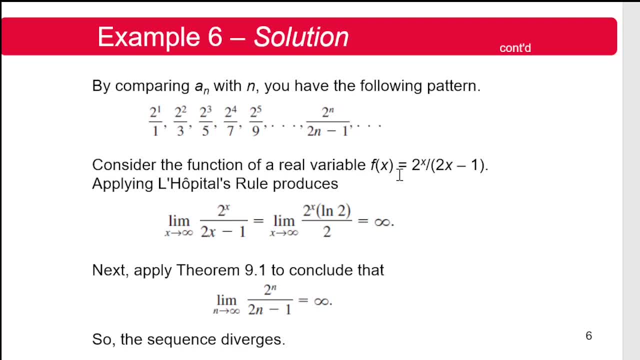 And then, after that, we can write the n-term As a function of a real variable denoted by f of x, which is 2 to the x over 2x minus 1.. And if you can recall the theorem 9.1,, we have to evaluate the limits of this function. 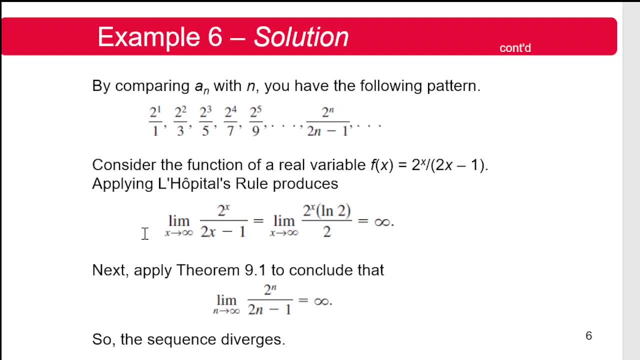 So to evaluate the limits of this function, we rewrite this in this notation as limits of 2 to the x over 2x minus 1, as x approaches positive infinity, And then we replace the x variable by infinity. So you have 2 raised to infinity over 2 times infinity minus 1 is infinity. 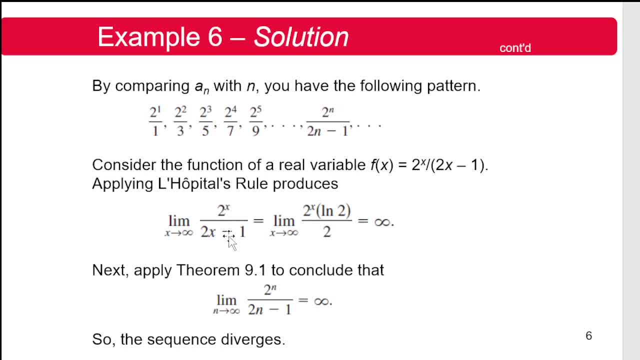 So the numerator and the denominator are both infinities, So you have infinity over infinity. And, if you can recall, in calculus these type of limits are indeterminate forms. So in this case, because the numerator and denominator are both infinity, So we can apply L'Hôpital's rule to evaluate the limits. 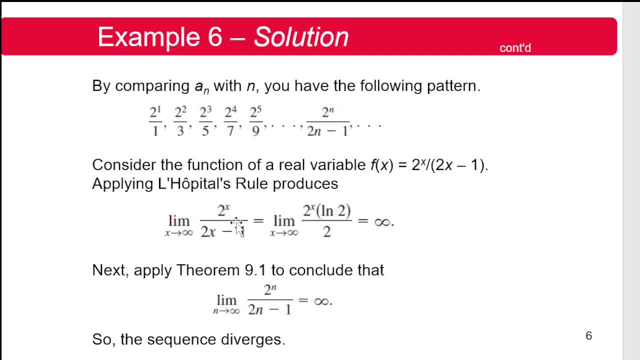 So differentiating the numerator and the denominator separately. if you can recall, the differential of 2 to the x is 2 to the x times the natural log of a, where a here is 2, all over the differential of 2x minus 1, which is 2.. 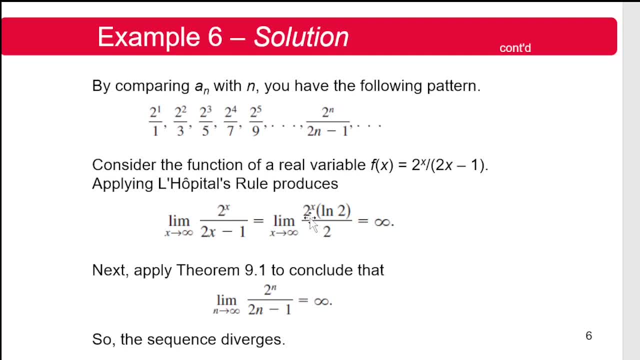 And then after that, by replacing the x variable by infinity, you have 2 raised to infinity times. the natural log of 2 is infinity. divided by any constant, 2 is infinity. So therefore the limits of this function- 2 to the x over, 2x minus 1, is equal to infinity. 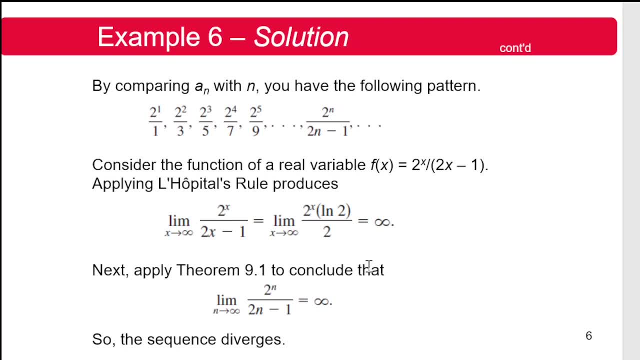 Then, by applying theorem 9.1,, we can now conclude that the limits of 2 to the n over 2n minus 1, as n approaches infinity, is infinity, Because the limits of this function is infinity. so the limits of the n term of the sequence, as n approaches infinity, is also infinity. 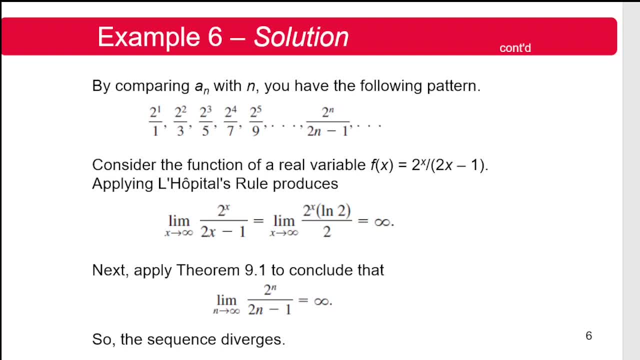 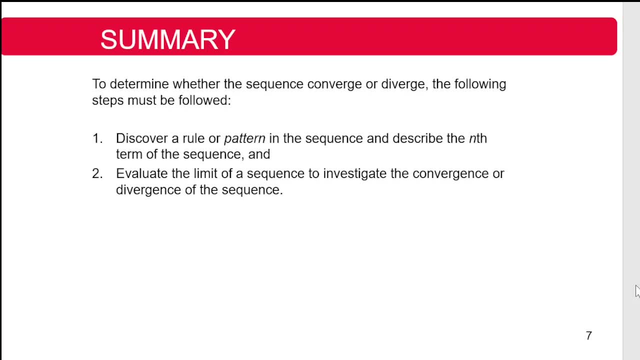 So this indicates that the sequence diverge. So, in summary, to determine whether the sequence converge or diverge, the following steps must be followed. That number 1, you have to discover a rule or pattern in the sequence and describe the n term of the sequence. 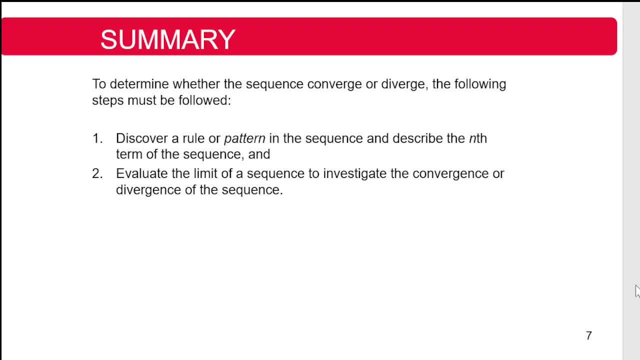 And then second, evaluate the limits of a sequence to investigate the convergence or divergence of the sequence. Okay, that's all for today. Thank you. 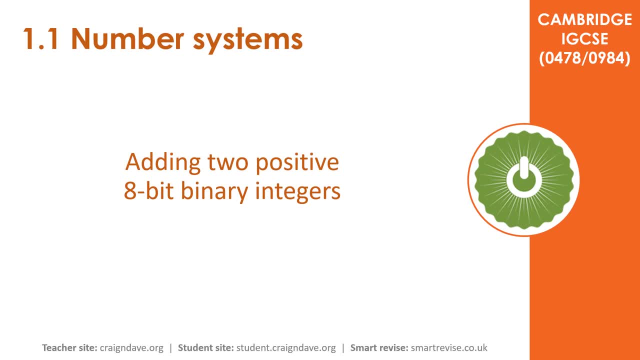 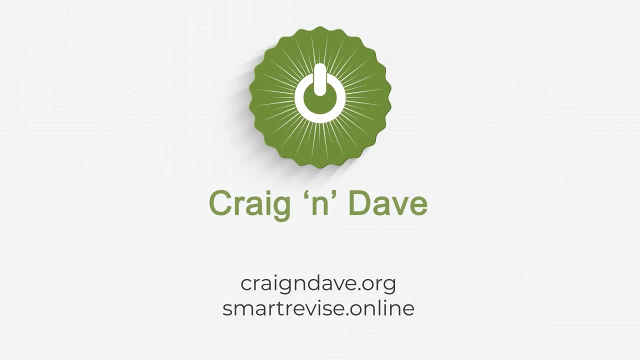 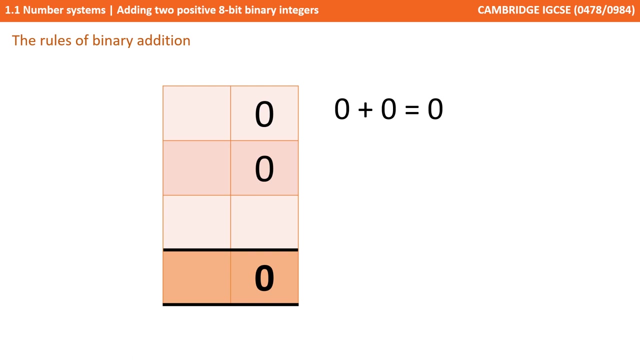 In this video we're going to look at how you add together two 8-bit binary integers. So before we work through some examples with you, let's just go over the basic rules for binary addition. So they're quite simple: a zero and a zero in binary equals zero. 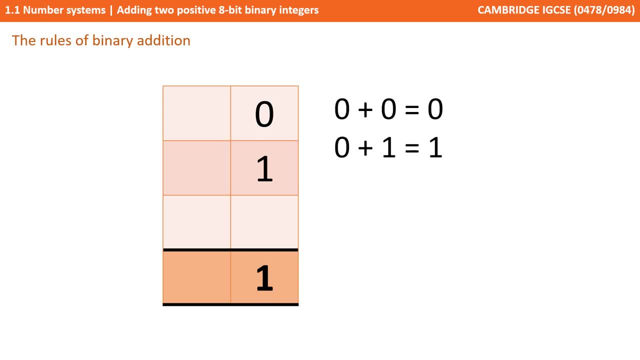 A zero and a one equals one. A 1 and a 1 can't equal 2 because we don't have a 2 in binary. so a 1 and a 1 in binary equals 0, and then we carry a 1 to our next column because 1, 0 in binary is the deanery number 2.. 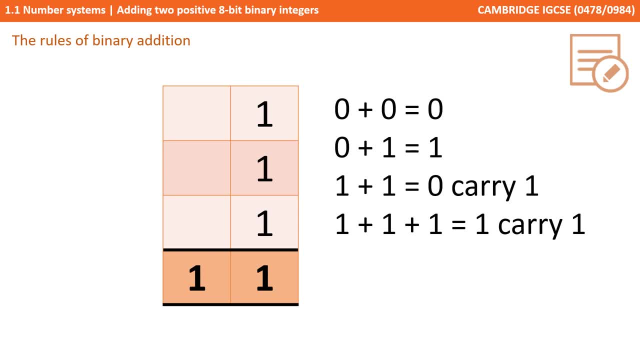 And finally, 1 plus 1 plus 1 in deanery is 3, but we can't have three, so it's one, carry a one. one. one in binary is three in denary, that's a one in the two column plus a one in the one column. now, these are the only four rules. 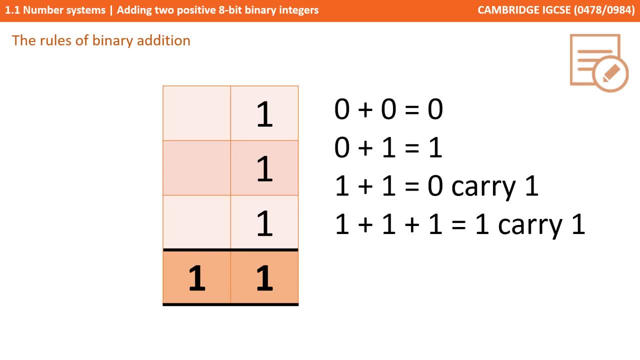 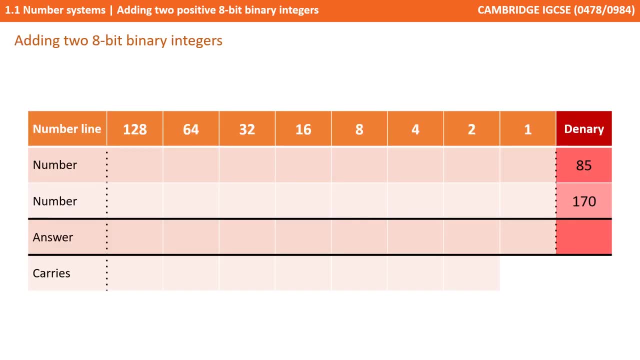 you're going to need at a GCSE level when adding together to 8-bit binary numbers. so let's work through some examples. so here we have a binary number line and we always suggest you write this out in the exam. you start with a one on the far.